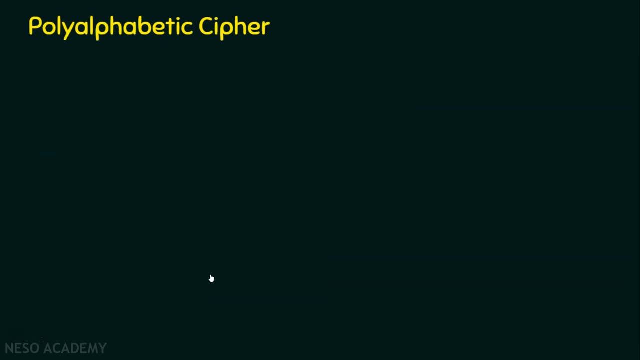 Let's dive into the topic of the day: the polyalphabetic ciphers. This polyalphabetic cipher is introduced to improve on the simple monoalphabetic technique. We have already seen the monoalphabetic substitution technique, where each letter can be randomly replaced by other letters. 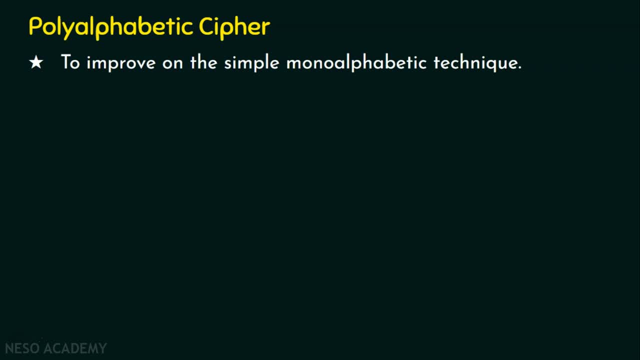 But the problem is that, say, in monoalphabetic substitution, if the plaintext letter A is mapped to Z, in all the occurrence of the plaintext letter A- Z will be the ciphertext. So it is vulnerable to attacks And in order to improve the playing text, letter A- Z will be the ciphertext. 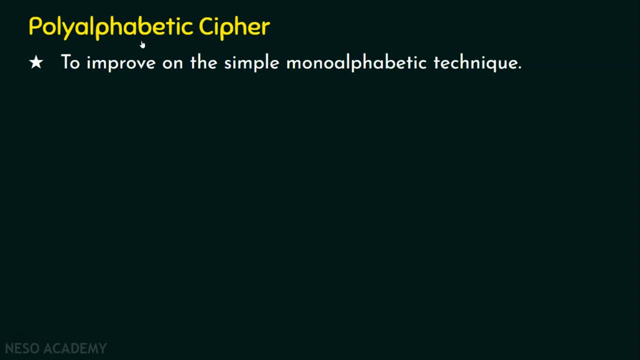 So it is vulnerable to attacks. In order to improve the monoalphabetic technique, polyalphabetic ciphering technique was introduced, And that's why it has been given with the general name polyalphabetic substitution technique. What are all the features of this polyalphabetic substitution technique? 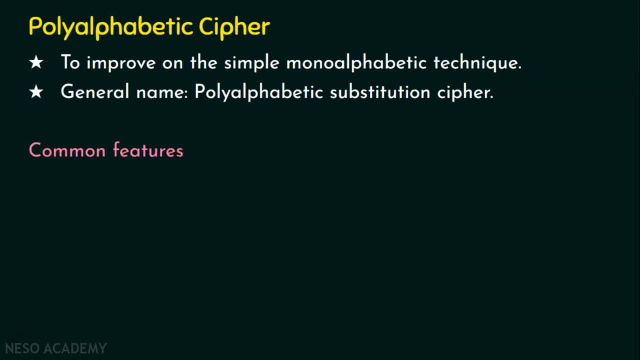 We have some common features. when you compare this with the monoalphabetic substitution technique, The common feature includes Number 1, a set of related monoalphabetic substitution rules is used. So in the monoalphabetic substitution we have a generalized rule. 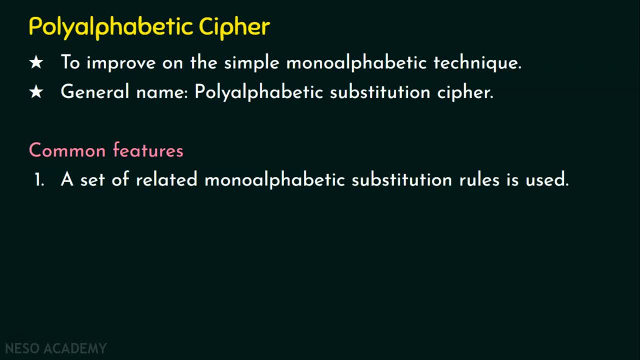 like what plain text letter will be replaced by what cipher text letter. Likewise, here, also a set of related mono-alphabetic substitution rules is used. And coming to the second feature, we have a key here, and this key determines which particular rule is chosen for a particular transformation or a given transformation. 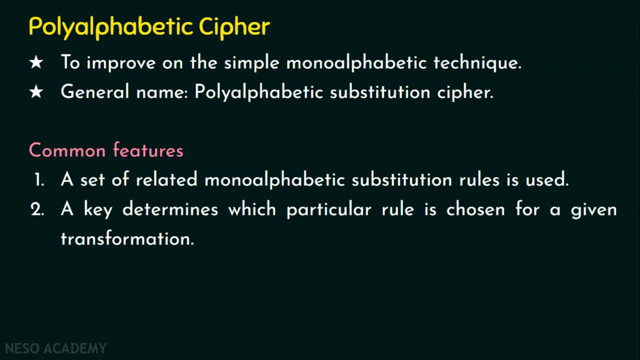 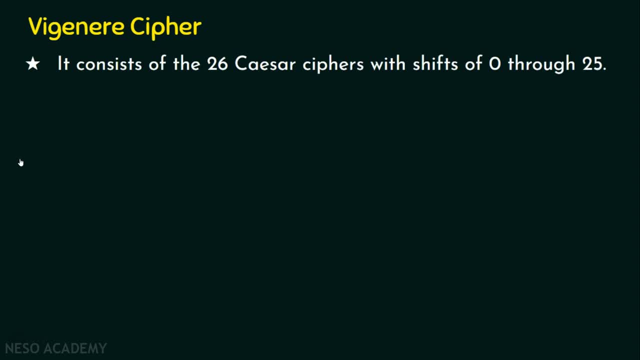 Anyway, we will understand the polyalphabetic cipher elaborately when we see an example. In this presentation, we are going to focus on the Wigener cipher. What is this Wigener cipher? Actually, this Wigener cipher consists of the 26 Caesar ciphers, which shifts 0 through 25.. 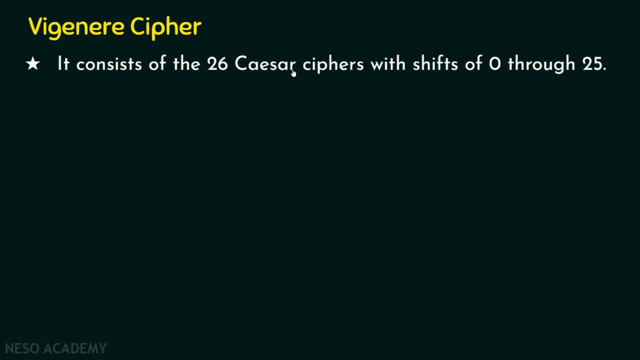 We have seen the first classical encryption technique, the Caesar cipher, where the key is fixed. the key is equal to 3 in Caesar cipher And we can see that the shifts between the plain text cipher text letters will be 3 always, Whereas in the Wigener cipher we are going to use 26 Caesar ciphers which shift 0 through 25.. 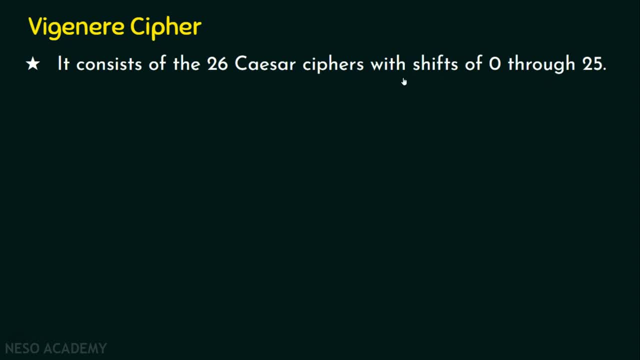 So don't worry, Don't worry about this point. When we see an example, you will understand this point clearly. So let's see the encryption process now. So, basically, the encryption process involves we are going to take the plain text letter which is at the ith position. 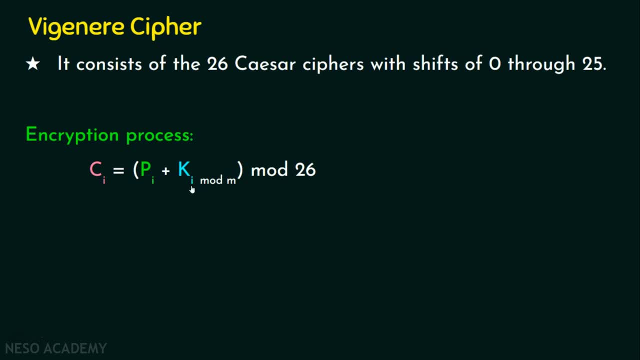 And this ith position plain text letter is added to the ith position. character of the key. And this summation is performed with mod 26,. whatever we get, that is the cipher text And this is the cipher text of the ith position, Because 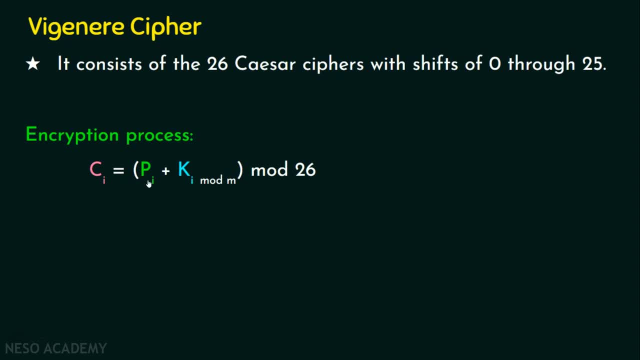 say, if you are encrypting the first plain text character, so the first plain text character and the first character in the key is added and it is performed with mod 26 and the result is the first cipher text character, Because i is equal to 1 in this example. 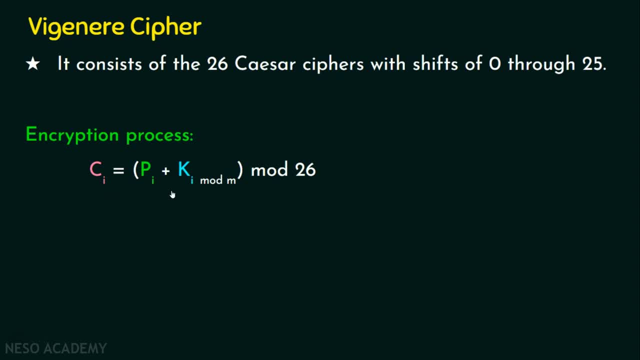 If i is equal to 2, it means we are taking the second character At the same time. this key- it can be a smaller key when compared to the plain text. For example, let's assume the plain text is having 2 characters. 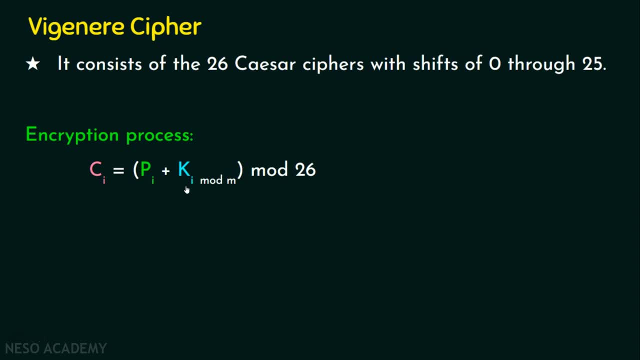 For example, let's assume the plain text is having 2 characters. For example, let's assume the plain text is having 25 characters And the key that we are taking is only 5 characters. How to add this? Because for 5 plain text characters, we have 5 characters in the key. 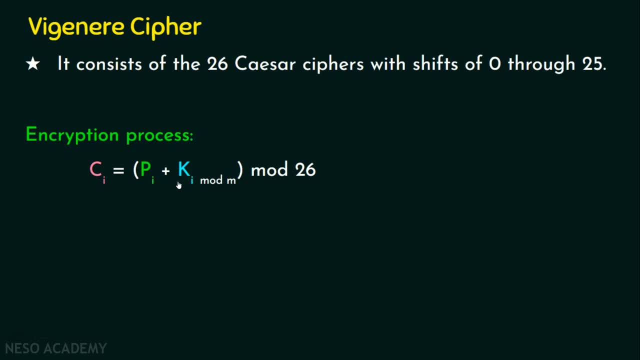 What about for other characters in the plain text, And that's why we are repeating the key. So I'll explain this when we see an example, So generally the encryption process of Vigenere cipher, where the plain text letter is added to the corresponding key character. 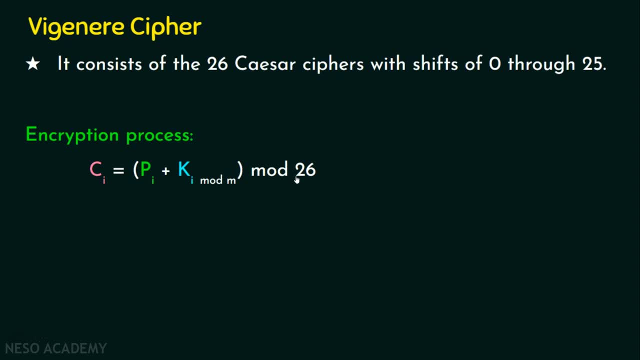 and then mod 26 is applied and the final result is the cipher. and then mod 26 is applied and the final result is the cipher. And then mod 26 is applied and the final result is the cipher, ciphertext, letter. and we know decryption is the reverse of encryption, where we are going to get 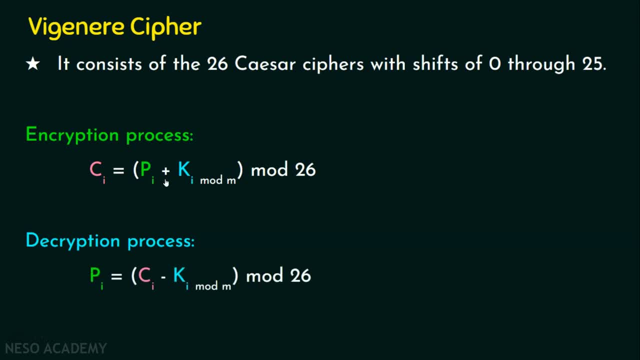 the playing text back. Plus operation is performed in the encryption and minus operation, that is, the subtraction operation, is performed in the decryption process. So whatever we get the ciphertext minus the key, mod 26 will give the playing text back. Let's see an example now. Say, let's take the key. 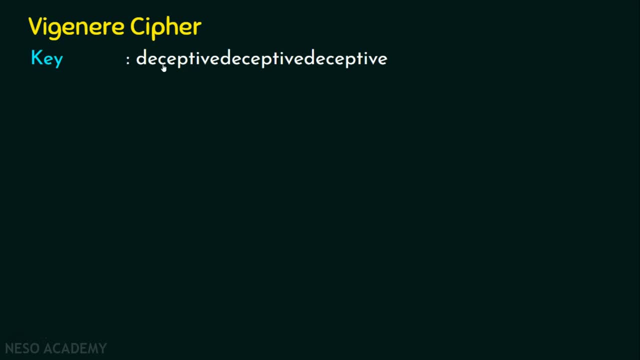 which is deceptive. Can you see? deceptive? Now, this is the key actually we have taken, but can you see? this key is repeated, deceptive again, and deceptive again. Why this key is repeated? Because the playing text may be a lengthy playing text, whereas the key may be a smaller key. So let's 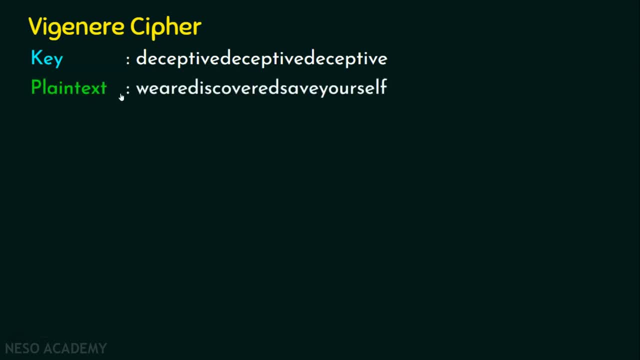 see that now. Yes, here in the playing text, we have the playing text as we are discovered: save yourself. So this is a bigger playing text, whereas the key is a smaller key, Deceptive. So what we are going to do is we are going to repeat the key as long as the message 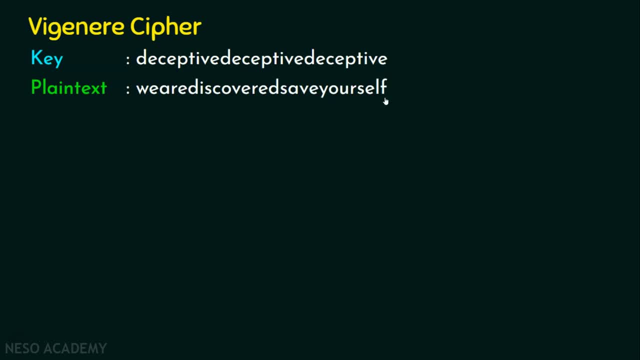 gets ended. So, for all the characters of the playing text, we need the key, Isn't it? Because we are going to perform the summation operation. So, for all the characters of the playing text, we are going to repeat the key as long as the playing text is reaching the end, and we obviously will be getting 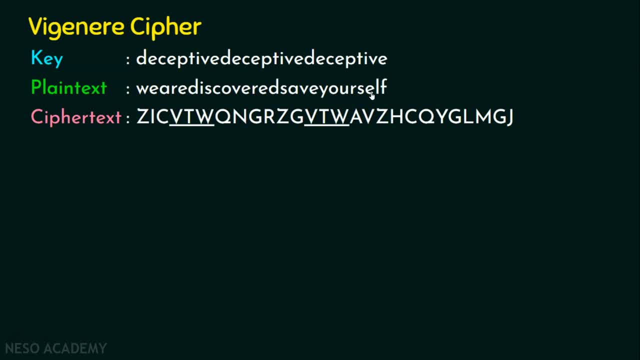 the ciphertext. So the ciphertext for this playing text we are discovered, save yourself with the key deceptive is this one. How did we get this? Let's see that now. So, in order to solve this problem, let's take a table like this: 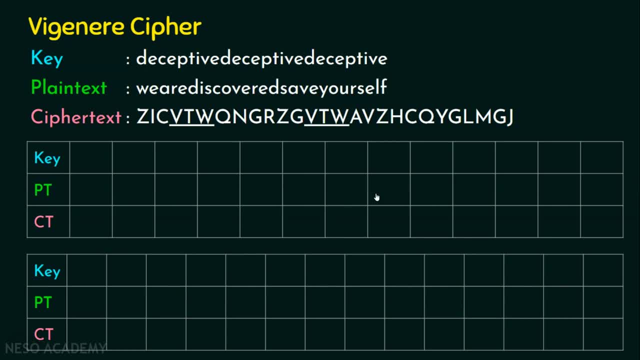 where I am going to put the key value here, the playing text character here and the ciphertext character here. Since we are having a bigger playing text, I am solving this in two tables. So what's the first step? We have the key right: Deceptive, As I already mentioned, this Vigenere cipher. 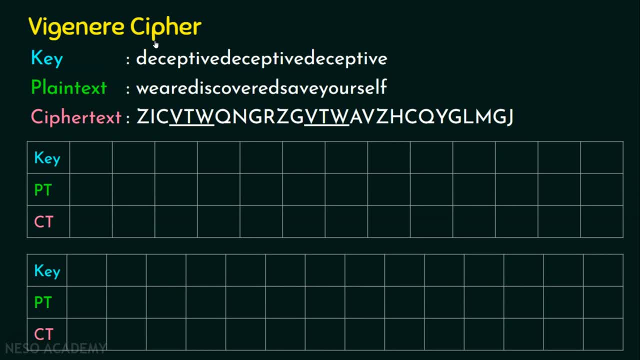 is a polyalphabetic cipher which uses Caesar cipher principle, So for every character we have numbers right. What is the number for D? If you are not sure about Caesar cipher, I request you to watch my previous lecture titled Caesar cipher, part 1.. 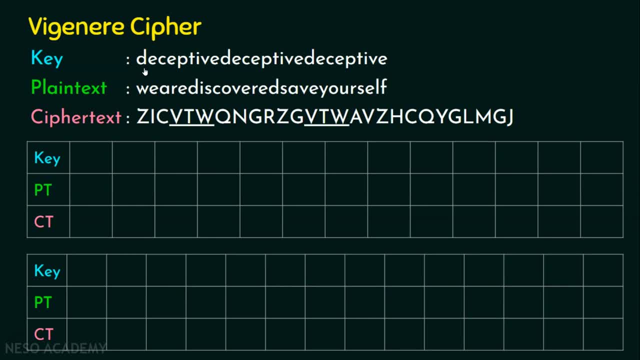 What is the number we use for the alphabet D in the Caesar cipher technique? 3, right, Because A is 0,, B is 1,, C is 2 and D is 3.. So D means number 3 and for E it is 4, right. 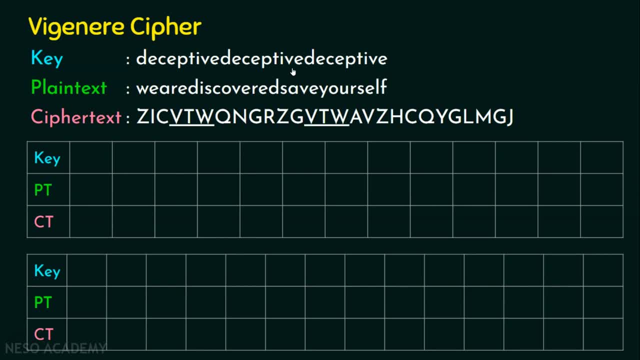 So for all the characters we have numbers. So for every character we have numbers. So for all the key letters we have equivalent numbers. I am just filling that equivalent numbers in this place. What do you mean by this? For D it is 3.. 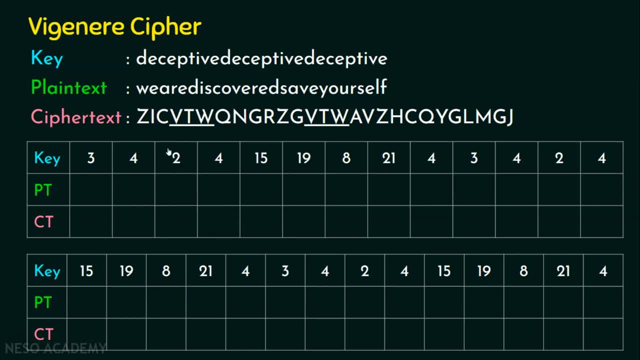 For E it is 4.. For C it is 2.. How 2?? Because A is 0,, B is 1,, C is 2.. For E it is 4.. For P it is 15.. 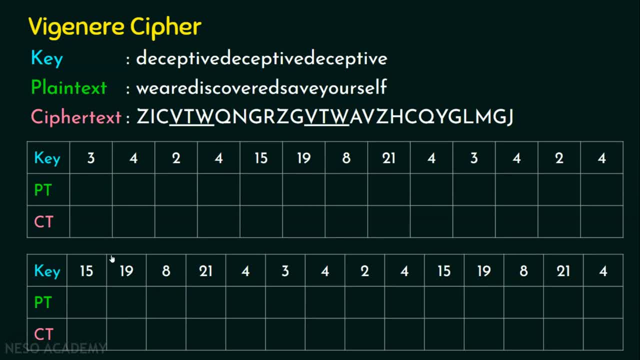 So for this entire keyword, I am just using its corresponding number on the first row. So we are done with the key part. Then we are going for the playing text part. In this playing text part we can see the playing text is: 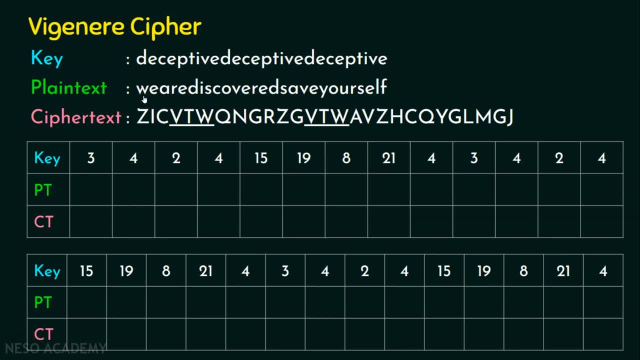 We are discovered. save yourself right. Let's focus on the first character, W. What is the number equivalent to W? It is 22.. What is the number equivalent to E? It is 4.. What is the number equivalent to A? 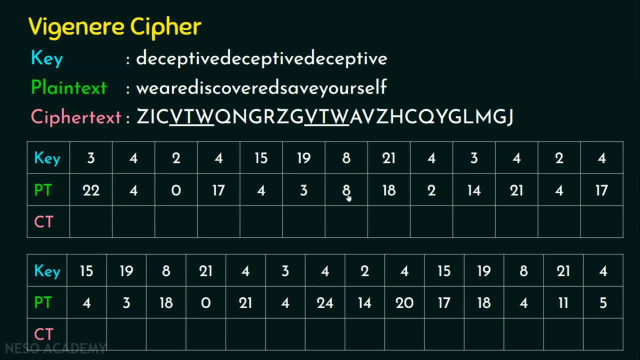 It is 0.. Likewise, we are going to assign the equivalent numbers in this row, That is, in the second row, Because second row is playing text and the first row is key And we are repeating the key as long as the message is. 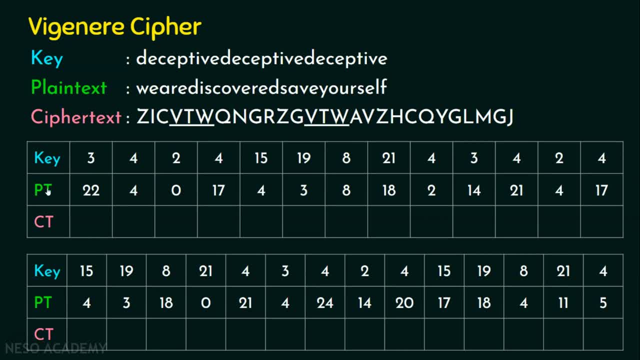 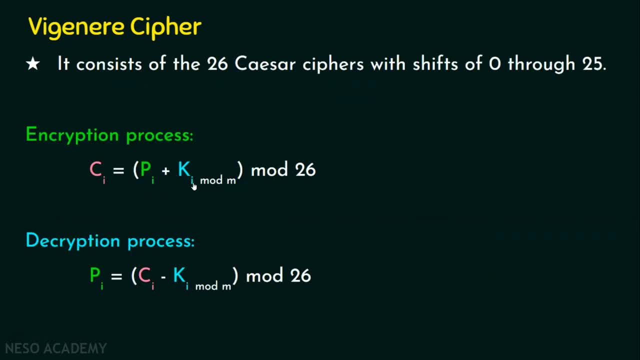 So we are done with the key part. Then we are going for the playing text part. So we are done with the key and the playing text. Let's revisit the formula. What is the formula for encryption? The letter in the ith position of the playing text is added to the letter in. 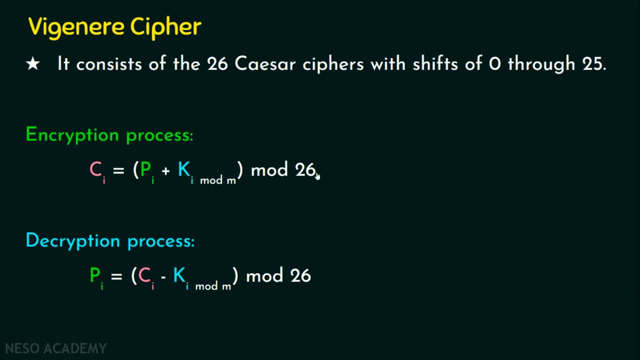 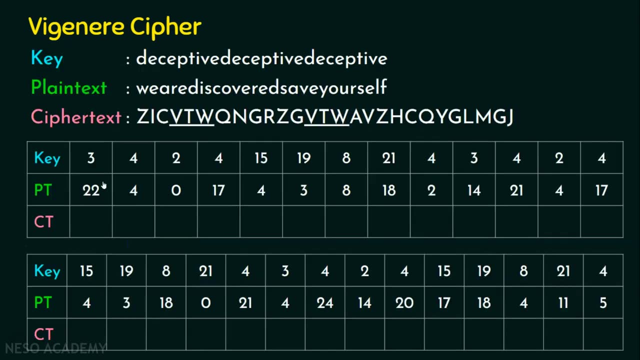 the ith position of the key, Then, whatever we get, perform mod 26.. And whatever we get is the ciphertext That is at the ith position itself. Let's see the problem now. So we are going to take the first position. 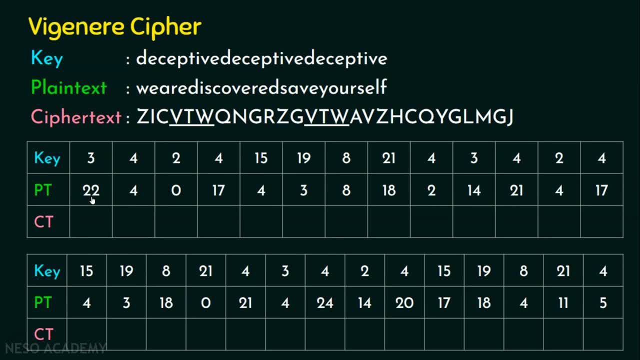 So the first position of the key is added to the first position of the playing text. So 3 plus 22 is equal to 25.. 25 mod 26 is equal to 25, only right, If you are not sure how to perform mod. 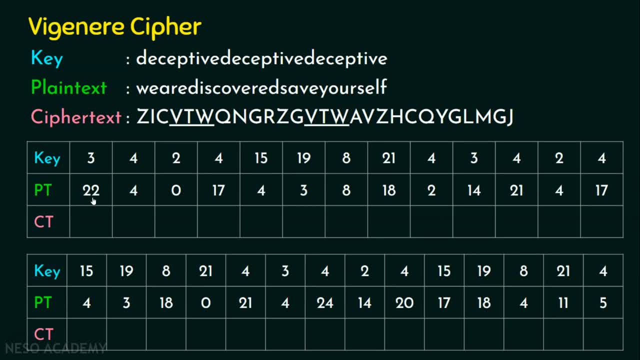 operation. I request you to watch my previous lecture, Caesar Cipher, where I have explained you how to do mod operation. So 3 plus 22 is 25.. 25 mod 26 is 25 only. So we are getting 25 as the ciphertext. What is the character equivalent to this? 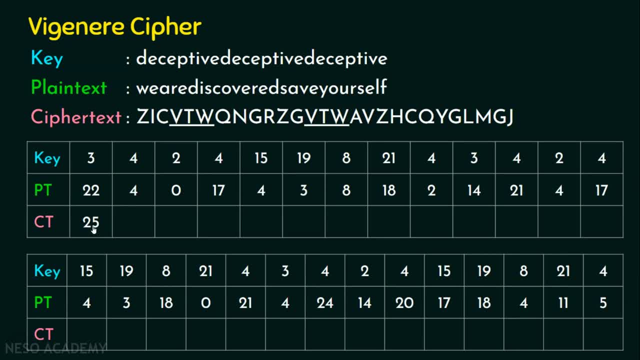 number 25?? It is z right, Because a is equal to 0,, b is equal to 1, and obviously, if you proceed like this, we get z is equal to 25.. So the ciphertext for this playing text, character w with the key value d, is z. 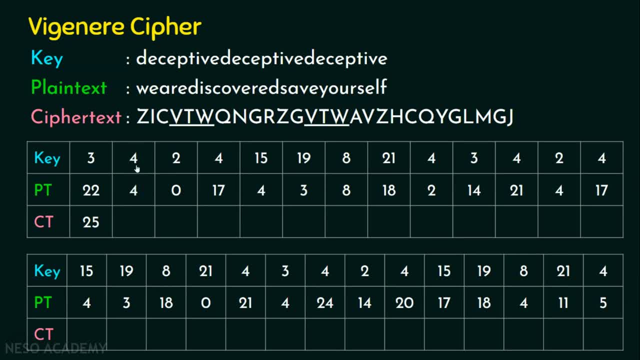 And what about the second playing text, letter encryption. So 4 is the key, 4 is the playing text. So 4 plus 4 is what 8.. 8 mod 26 is 8 only. So 8 means which character has the number 8?? 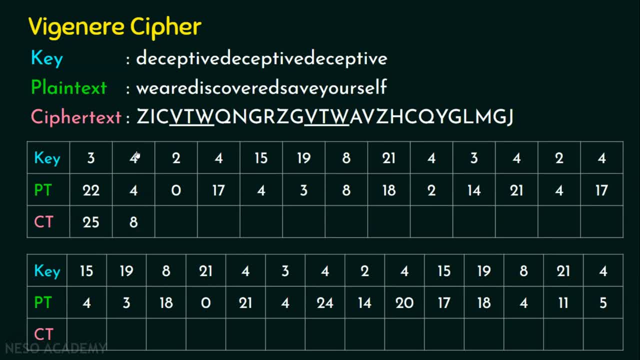 i is the alphabet that has the number 8.. Let's now move on to the third playing text letter. which character has the number 8?? i is the alphabet that has the number 8.. Let's now move on to the third playing text letter. which character has the number 8?? 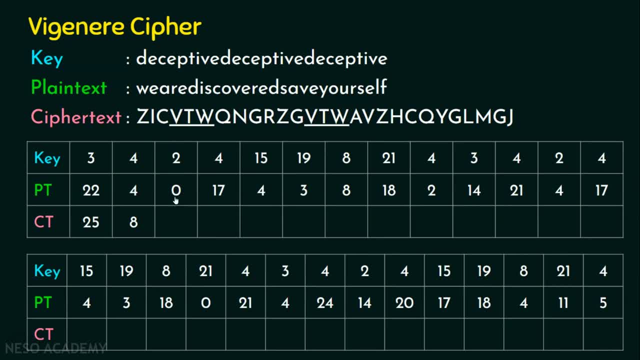 i is the alphabet that has the number 8.. Let's now move on to the third playing text letter, which is 0 here. So 2 plus 0 is 2.. 2 mod 26 is 2 only right. 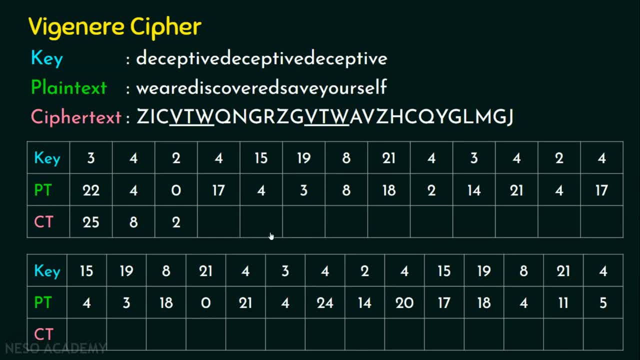 So likewise, we need to carry out the same addition operation, mod 26, for remaining playing text letters. I have completed this. Let's take this scenario: This is 21.. 21 plus 18.. We will get 39, right. 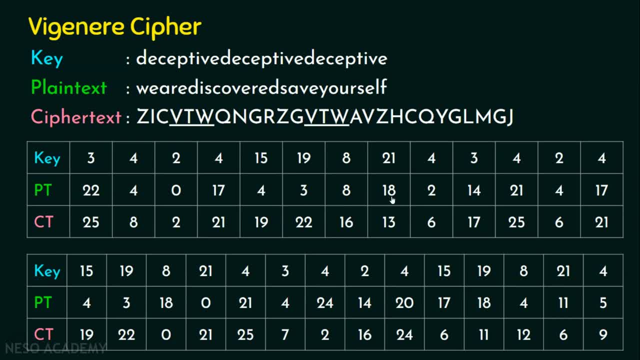 So 39 mod 26.. If you perform 39 mod 26,, what will be the remainder 13, right? So 13 is the number for the playing text, letter 18 and the key value 21.. So the character equivalent to the number 13 will be the cipher. 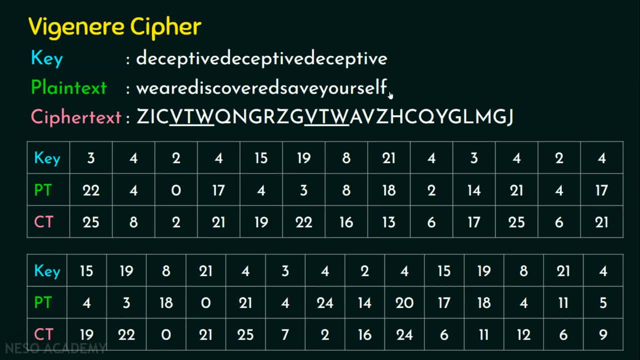 text letter. So this is how Vigenere cipher operates. Suppose if you still have playing text here, then repeat the key: deceptive, deceptive, deceptive, as long as the playing text letters are reaching the end. And this is about the Vigenere cipher. 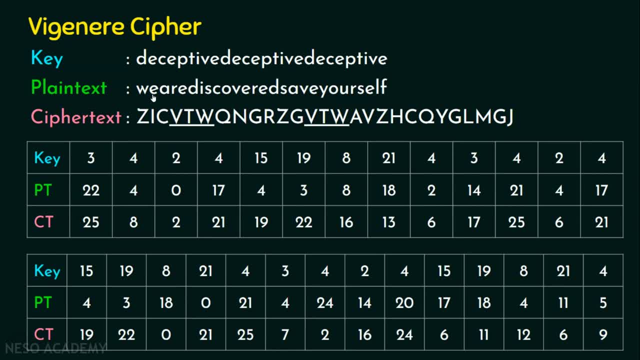 Let's see the security aspects now. Here the playing text letter e is encrypted as i here, right, Coming to this place. this playing text letter e is encrypted as t here. Why there is a change? Because we don't know what is the character from. 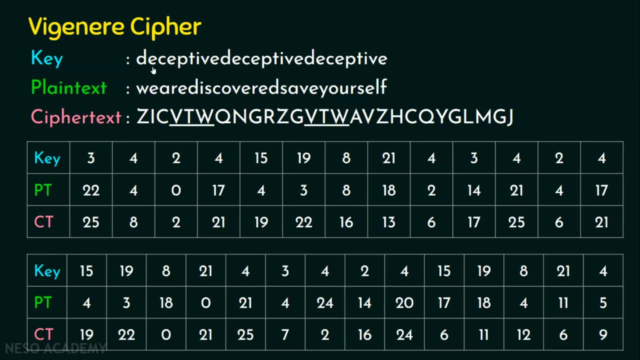 the key For this e the character. what we get from the key is e only, Whereas for this e the character we get from the key is p. So the key value is differing and that's why this is also a multi-letter encryption. So for the same playing text letter, we can't expect the same. 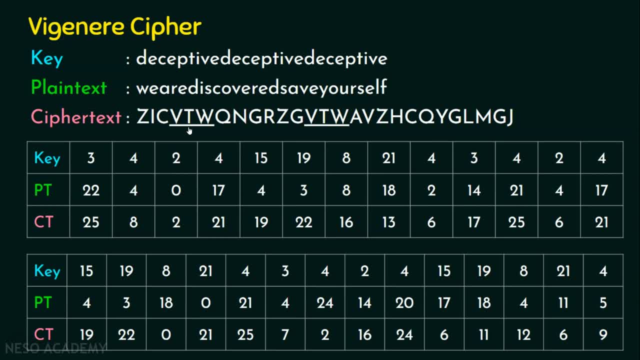 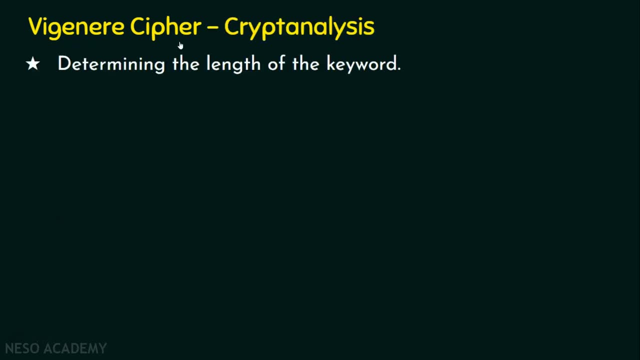 cipher text letter, Whereas in mono-alphabetic cipher, wherever the playing text letter appears has a corresponding cipher text and throughout the entire message the same scheme is followed. Let's now see the cryptanalysis on the Vigenere cipher. The important thing about the Vigenere cipher is determining the length of the key, Because 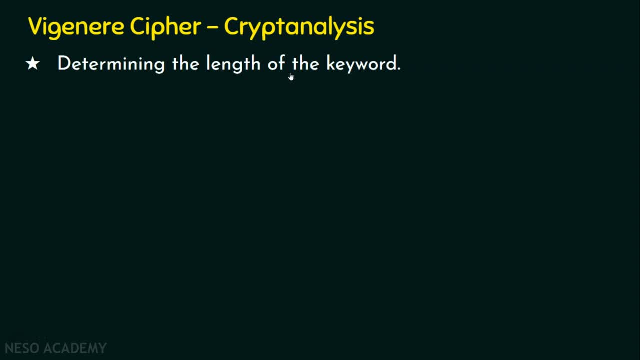 the key is going to be repeated, and determining the length of the key is a very, very important aspect as far as cryptanalysis is concerned. And the second one is the key and the playing text letters share the same frequency distribution of letters. That is, a statistical technique can be applied. 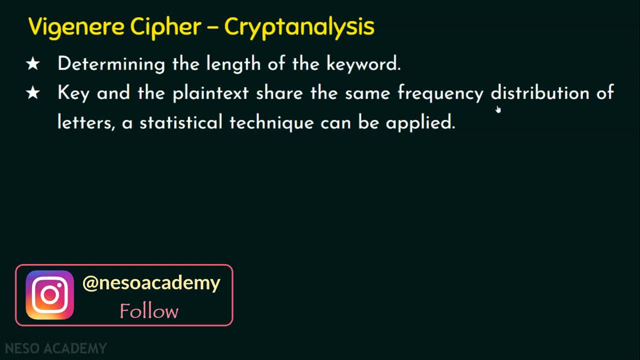 We know that English letter frequency distributions- both the key and the playing text share the same frequency distribution, And these two points are the important points that should be considered for cryptanalysis when we deal with Vigener cipher. Before we conclude, let's see the AutoKey system. 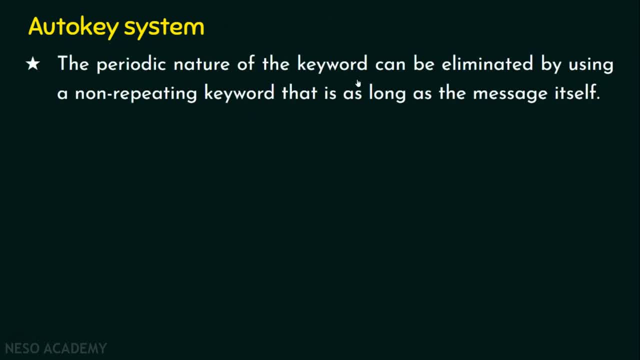 Actually, this AutoKey system means the periodic nature of the keyword can be eliminated by using a non-repeating keyword that is as long as the message itself Say. in the example what we have seen, we can see the keyword is repeating throughout the message, right? 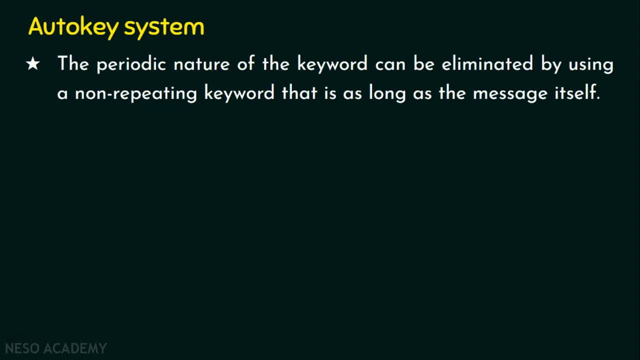 Deceptive, deceptive, deceptive, and it goes on as long as there is a message. If the attacker is able to determine the length of the key, then he can identify that this keyword is repeated, isn't it? So instead of that, what we can do is we are going for an AutoKey system. 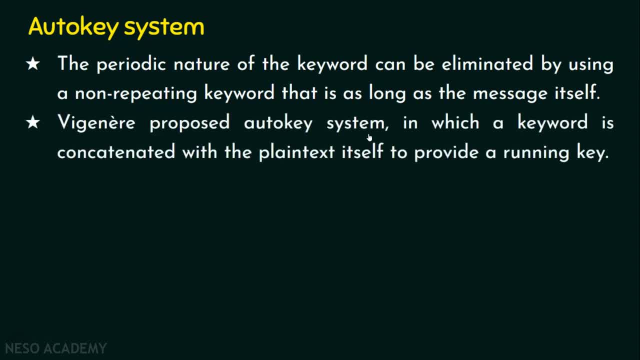 which was actually proposed by Vigener, and in this AutoKey system, where a keyword is concatenated with the playing text itself to provide a running key. We will see an example. then this point will be easy for you to understand. Say: we have a keyword, right. 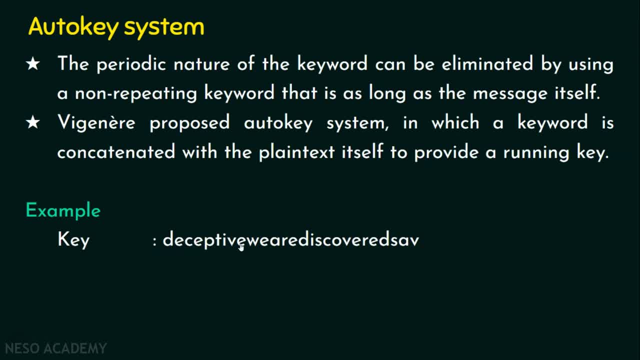 The keyword is what Deceptive. After this keyword, we are going to take the playing text itself as the key. Can you see here? We know the playing text is: we are discovered, save yourself. Now we are taking a key here and we are not repeating the key. 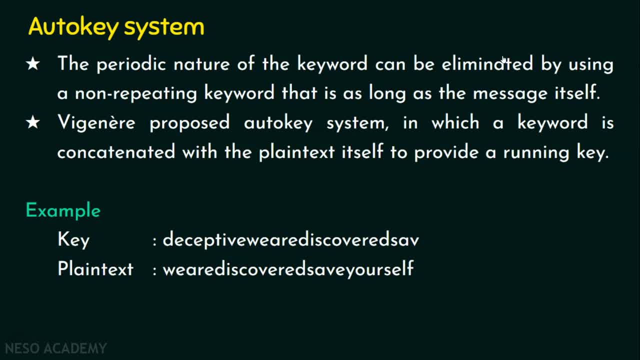 After the key ends. we are taking this playing text itself so that we are eliminating the repeated keywords, So the keyword deceptive is not repeated throughout. Using this, we get the ciphertext by applying the same logic, what we have seen in the Vigener cipher. 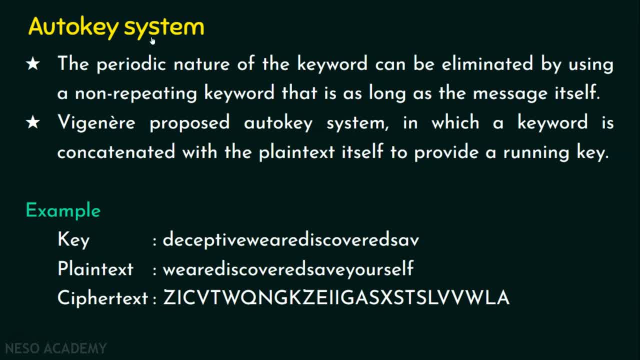 It seems that this AutoKey system offers better security when compared to the simple Vigener cipher. I hope now you can understand point number 1 and point number 2 clearly. We are eliminating the repeating keywords, That is, we are going to introduce. 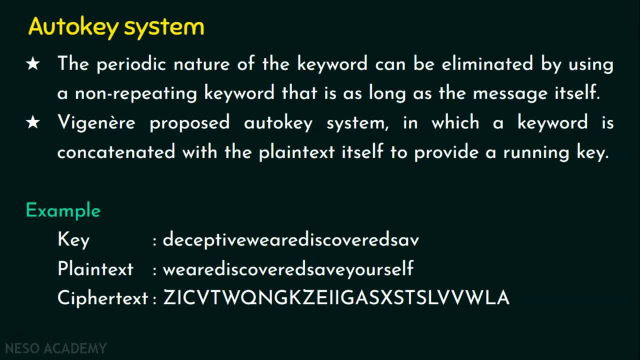 a non-repeating keyword. How it is introduced. We have a keyword deceptive. With this keyword, we are concatenating the message itself so that it becomes a non-repeating keyword. And that's it, guys. I hope now you understood the polyalphabetic substitution cipher.